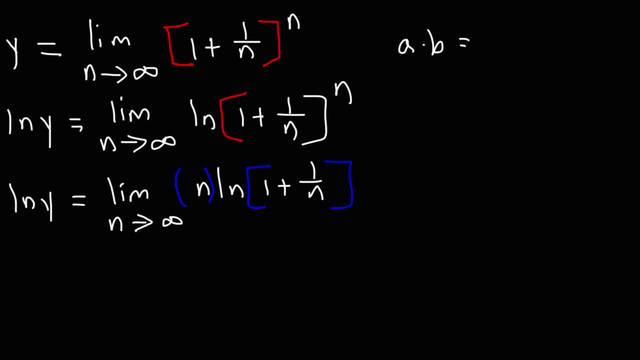 And here's how we can do that. For instance, a times b is equal to b divided by 1 over a. So here we have a product of two expressions. Now we have a quotient of two expressions. You can illustrate this with real numbers. 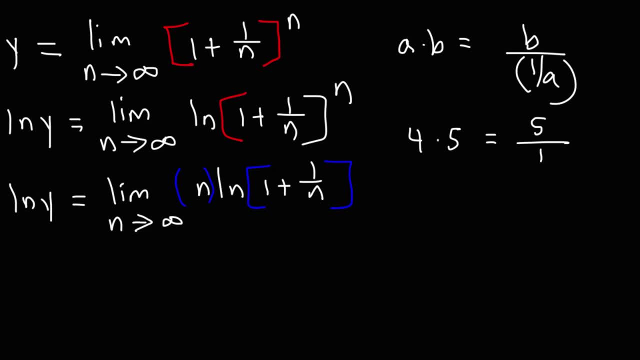 4 times 5, which is 20, is equivalent to 5 divided by 1 fourth. They both equal 20.. So, based on that, we're going to convert this expression from n times the natural log of 1 plus 1 over n. 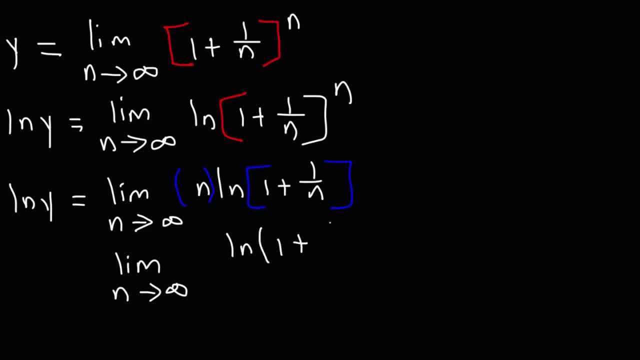 to ln. 1 plus 1 over n. divided by 1 over n, They're mathematically equivalent. So now, in this format, we could use something called L'Hopital's Rule, which is useful for evaluating limits that approach infinity. 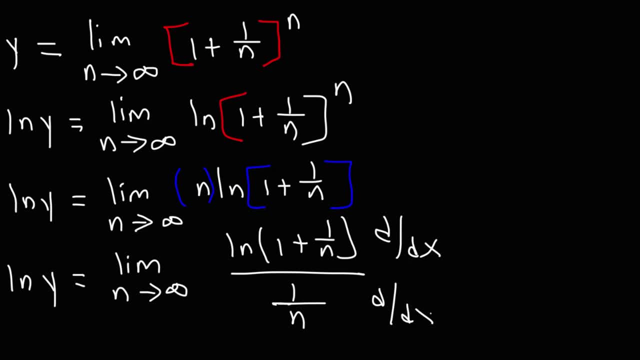 So we're going to take the derivative of the top and of the bottom. Let's start with the numerator. The derivative of the natural log of u is equal to u' over u. So since the u variable is going to be the stuff inside of the natural log function, 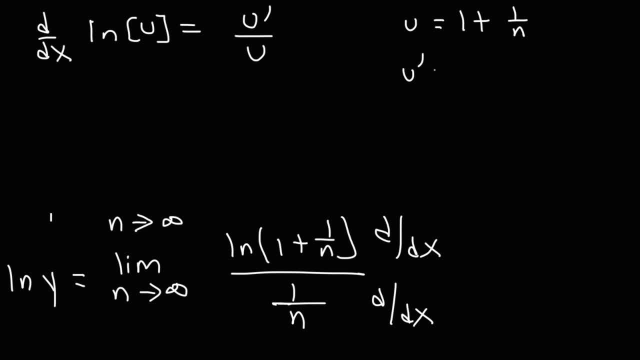 that's going to be 1 over n. So since the u variable is going to be 1 plus 1 over n, u' is going to be the derivative of that expression. The derivative of 1 is 0.. Now the derivative of 1 over n. 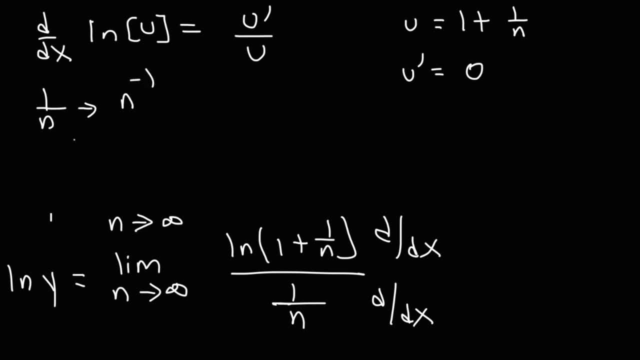 first we need to rewrite that as n to the minus 1.. And then we need to use the power rule, So it's going to be negative 1, n to the minus 2.. And then we can rewrite that as negative 1 over n squared. 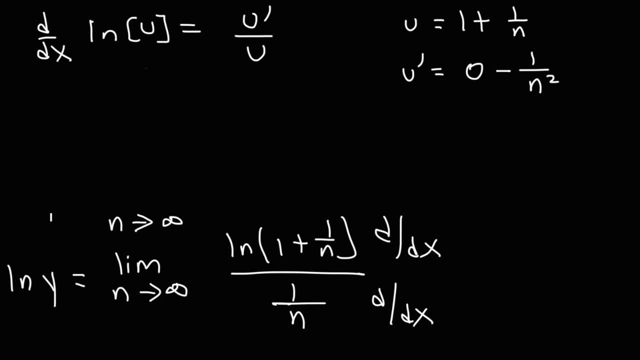 So using the formula u' over u, we're going to have: Lny is equal to the limit, as n goes to infinity, And the derivative of that expression is going to be u' which is negative: 1 over n squared divided by u. 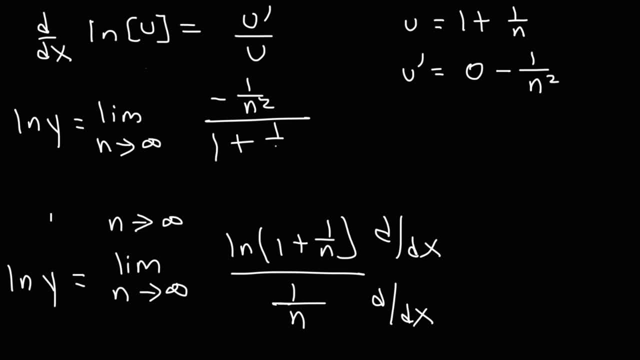 which is what we see here. That's 1 plus 1 over n, And all of that is divided by the derivative of 1 over n, which is, this again, negative: 1 over n squared. Whoa, what just happened. 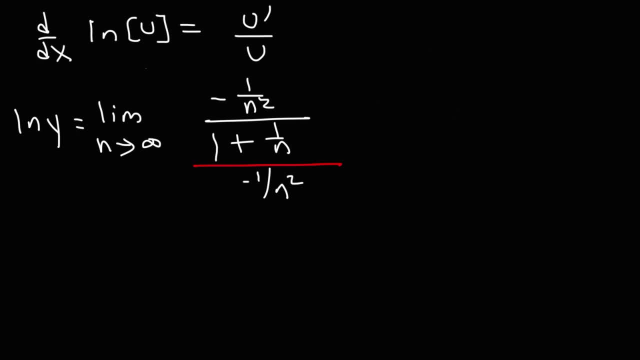 Now, let's get rid of that. Now, the next thing that we need to do is cancel the two negative signs. A negative divided by a negative sign is a positive sign, And then we can multiply the numerator by n squared and the denominator by n squared. 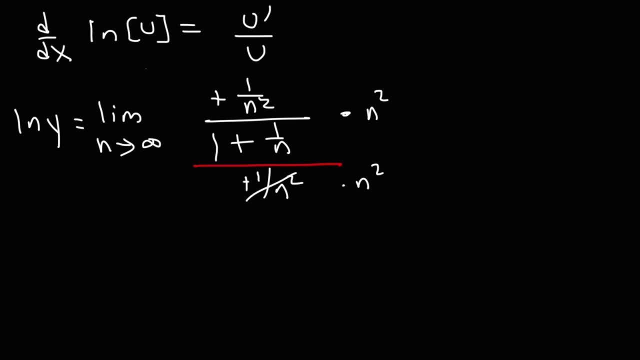 So 1 over n squared times n squared, this is just 1.. And this becomes 1.. So in the end we're going to get the natural log. of y is equal to the limit, as n goes to infinity. This is 1 divided by 1, plus 1 over n. 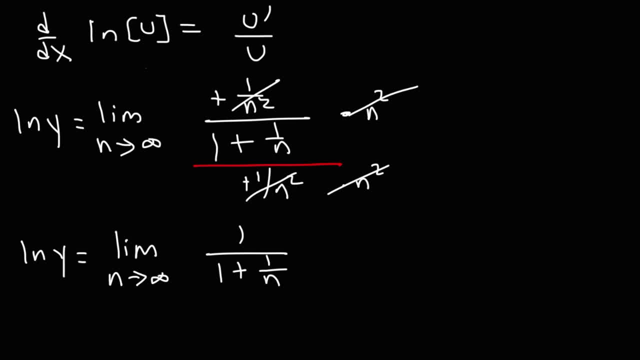 All divided by 1, which we don't really need to write that. So this is the expression that we now have. Now, as n goes to infinity, what happens to 1 over n? Let's say n is 10.. 1 divided by 10 is 0.1. 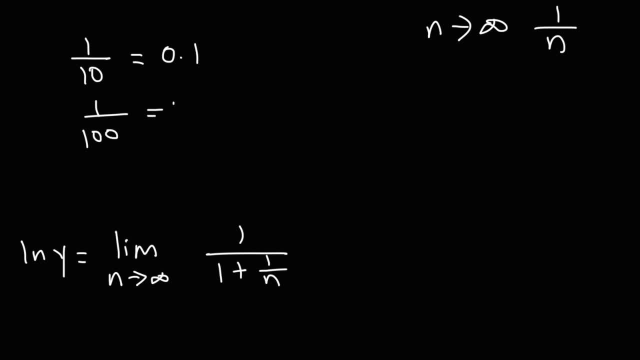 If n increases to 100, 1 divided by 100 is 0.01.. As n increases to 1,000, 1 divided by 1,000 is 0.001.. As n gets larger and larger, 1 over n gets smaller and smaller. 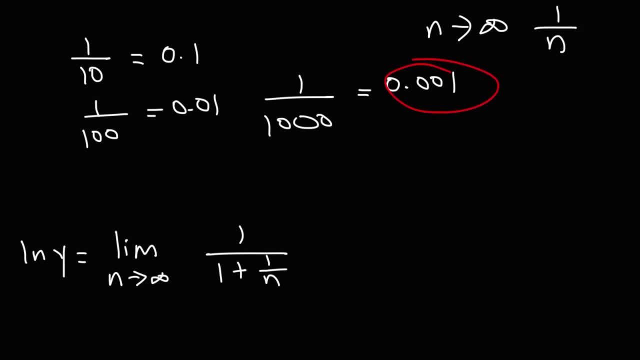 As you can see, it's getting close to 0.. So, as n goes to infinity, 1 over n approaches 0. So, applying this limit expression, we can replace 1 over n with 0. So we're going to have: 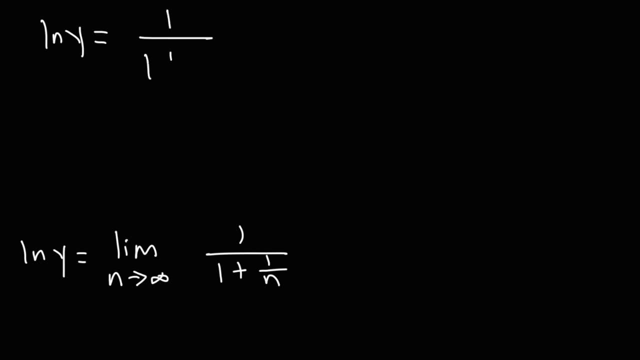 ln y is equal to 1 over 1 plus 0, which is basically 1.. So the natural log of y is equal to 1.. Now the base of a natural log function is equal to e. That's important because that's going to help us. 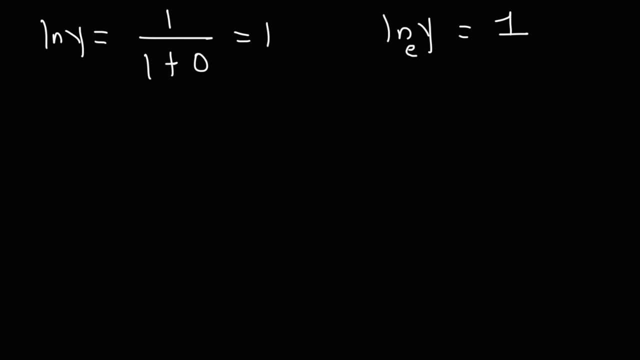 get the answer that we need. Here's a property of logs that you need to be familiar with: Log base a of b, let's say that's equal to c. To convert this from a logarithmic expression into an exponential expression, here's what you can do. 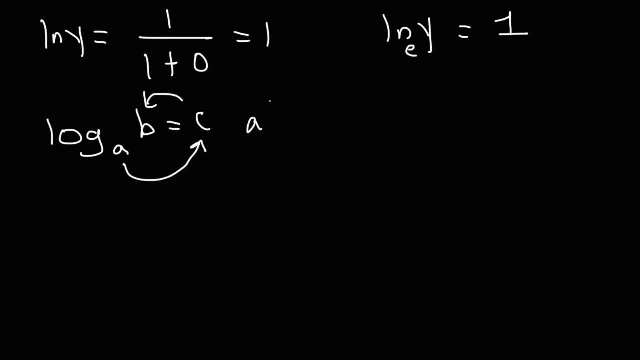 a raised to the c is equal to b. Now, applying that same process to the expression that we have in the upper right corner, we could say that e raised to the first power is equal to 1.. So therefore, y is equal to e. 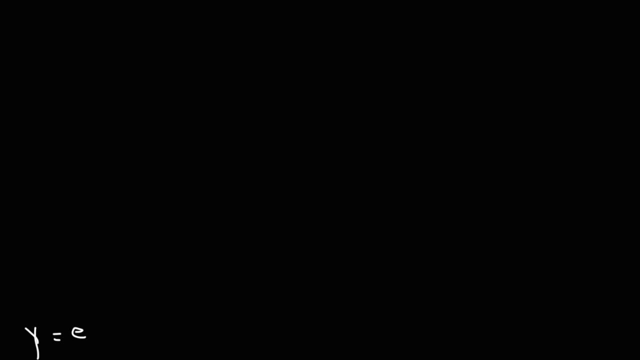 Now, going back to the original problem where we had this, we said that y was equal to the limit, as n goes to infinity, of 1 plus 1 over n Raised to the n, Because that's equal to y and y is equal to e. 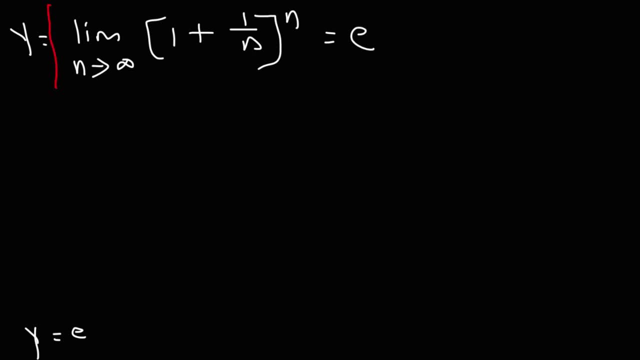 this limit expression is equal to e. So this right here is the answer to the problem. So that's how you can get the number e. e is equal to 2.718281828.. And then that continues on. We can plug in numbers to get this result. 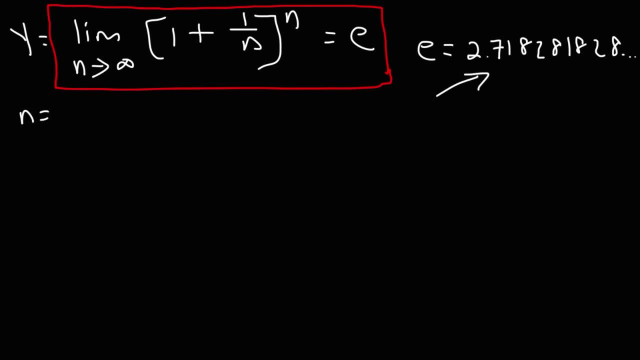 For instance, let's make n equal to a large number, Let's say 1,000.. So if you type this in your calculator, 1 plus 1 over 1,000, raised to 1,000, this is what you're going to get. 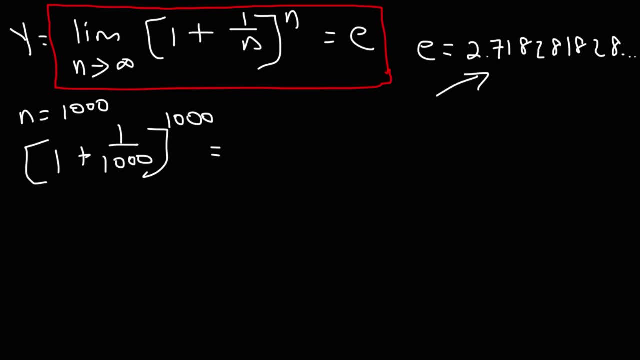 You're going to get 2.716923932.. Which is close to this answer, but not quite. Now let's increase n from 1,000 to a million. A million is basically 1 times 10 to the 6.. 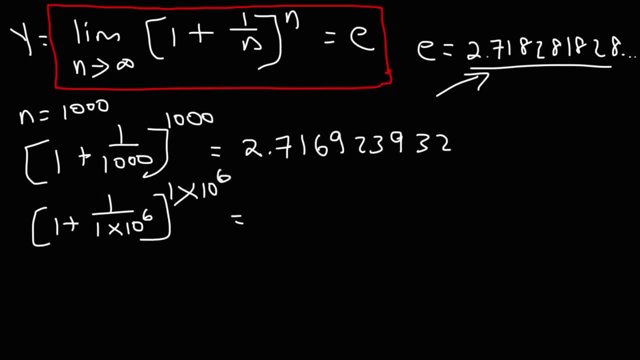 It's easier to type it that way. So if you plug in this number, you're going to get 2.718280469.. So this is really getting close to e. Now let's try one more. Let's try a billion. 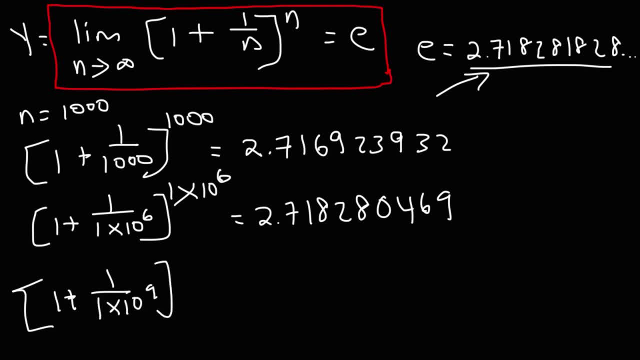 A billion is 1 times 10 to the 9.. So this is a very large number, And this will give you, at least according to my calculator, 2.718281827.. So the only thing that's different here is the last 8 and the last 7..